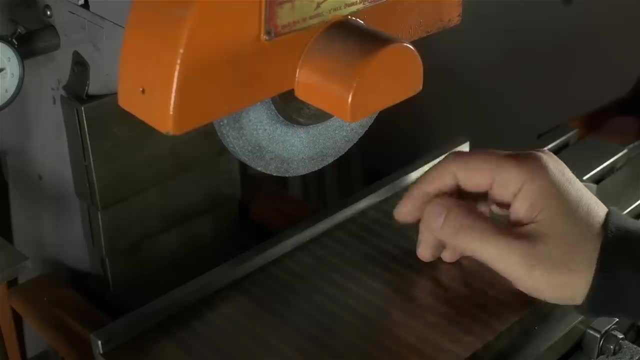 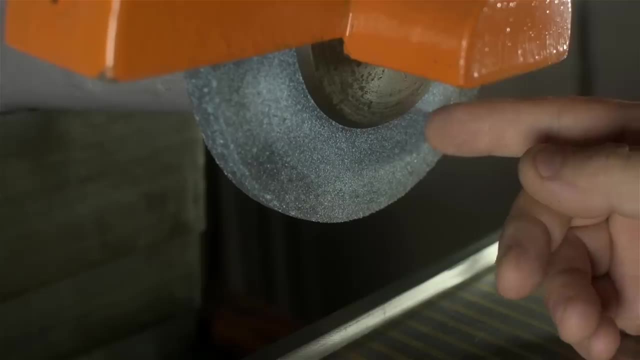 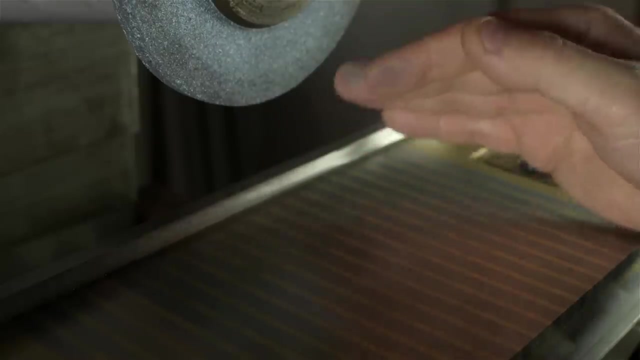 mentioned on this channel. It goes a little something like this: What they're asking, in not so many words, is: if the wheel wears down as it's doing its thing, how on earth does a surface grinder get such flat parts And, by extension, why isn't the part slightly tapered? 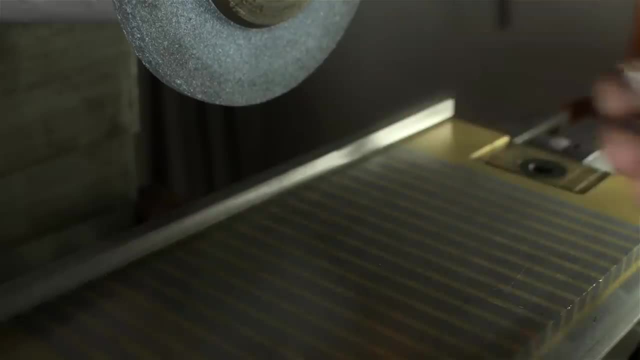 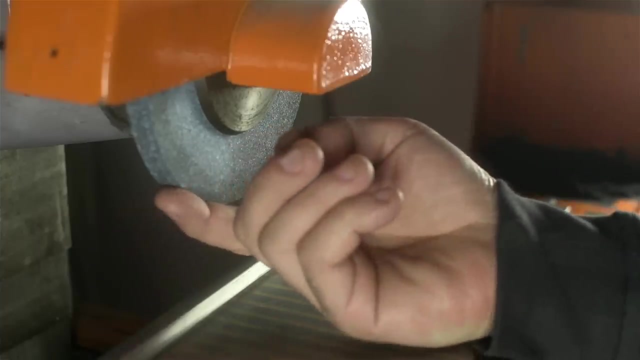 back to front, The premise being that the wheel wears by the time it makes it across the surface. Those are great questions, Natural questions. I assume come from years of people grinding grooves into the face of the wheels on their bench grinders. But what might really blow your minds is that surface grinder wheels are actually 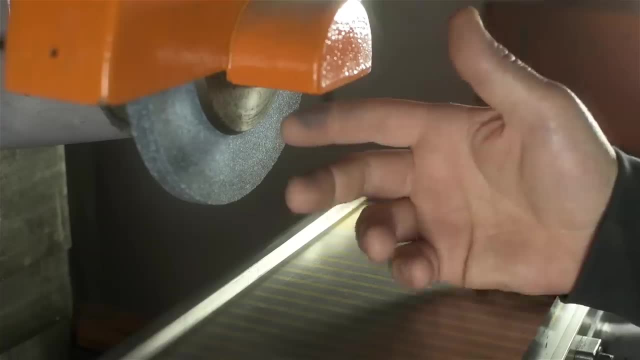 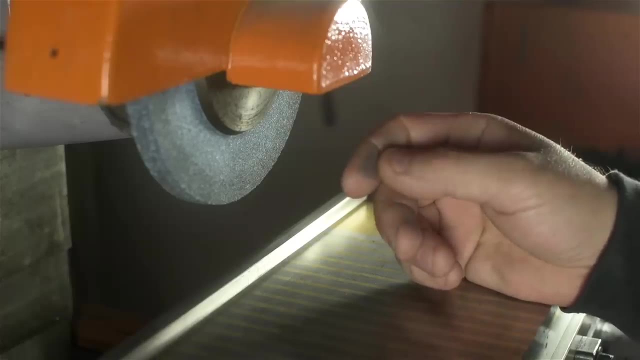 softer than bench grinder wheels. I mean, they don't have to be Depends on what you're grinding, But generally for hardened steel, which is the brazen detra for surface grinders, the wheels will generally be softer, Though, frankly, even hard and soft aren't that black. 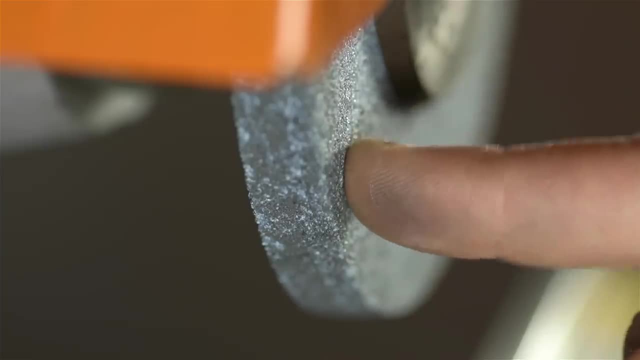 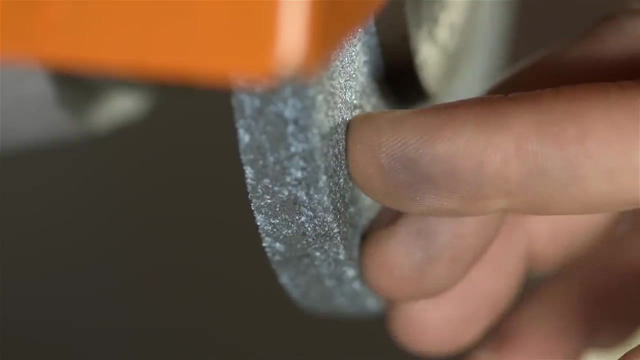 and white. when it comes to grinding wheels, These things can get complicated. Just do a little bit of grits: What the grit actually is made of, What the matrix is, How hard that matrix is, How friable it is, What color and flavor it might be. Honestly, it's worse than making heads or tails. 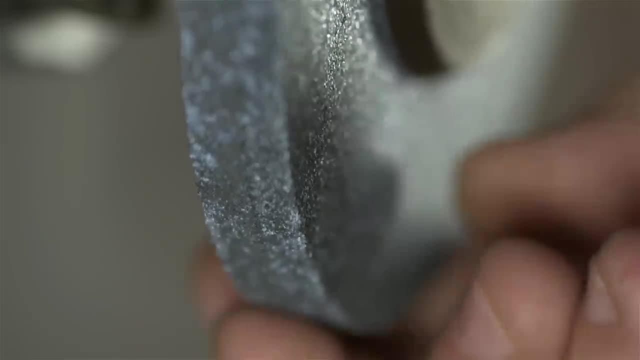 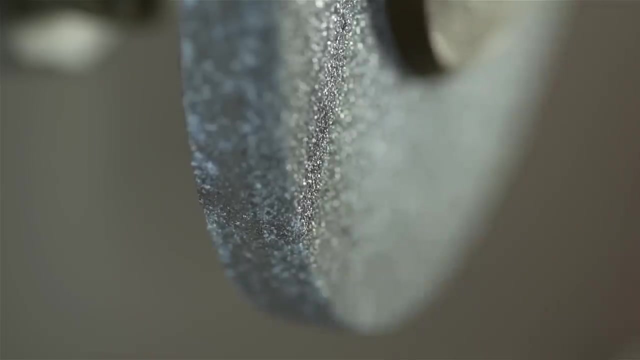 of insert tooling. Let's have a close look at this wheel, In particular the cutting face. You see all that chromatic aberration. See how it's all dirty and loaded up with metal. That right, there is the raisin. We got burn marks on the part. Let me dress it and I'd like you to keep a close eye. 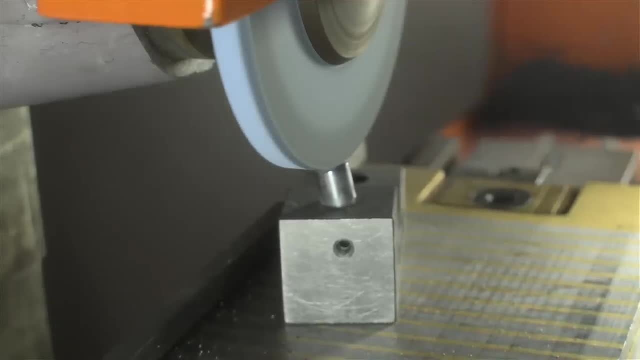 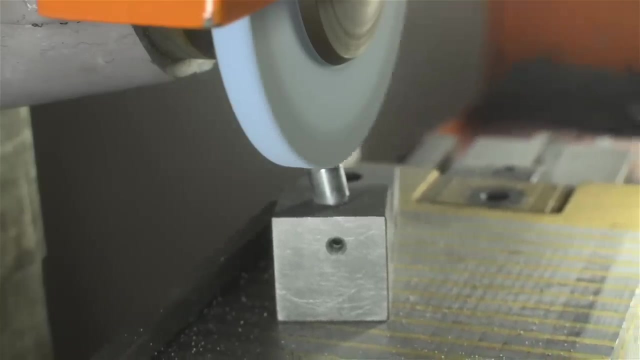 on the fresh cutting face as it develops. I'm using a little diamond nib to break down the glazed surface to reveal new sharp particles in the wheel. See how it's, cleaning the back part first and the new face is developing back to front. Well, your intuition is correct: The wheel does break down, of course, eventually. 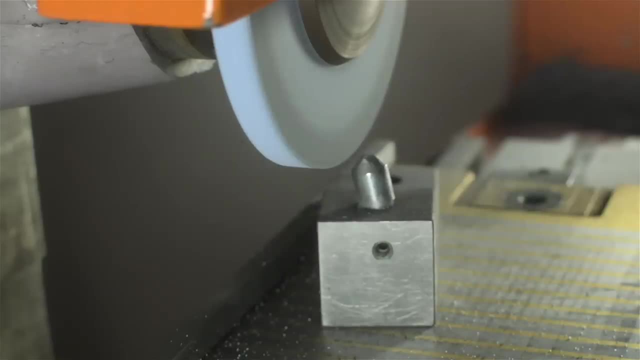 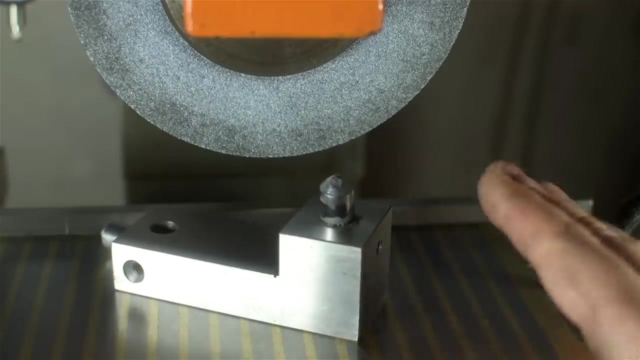 picking up a small taper front to back, But maybe not as you'd expect. Okay, one minute Before I put this away, a little safety detail I want to point out, And I do realize at this point we're three tangents deep in the wheel, So I'm going to go ahead and cut this off. 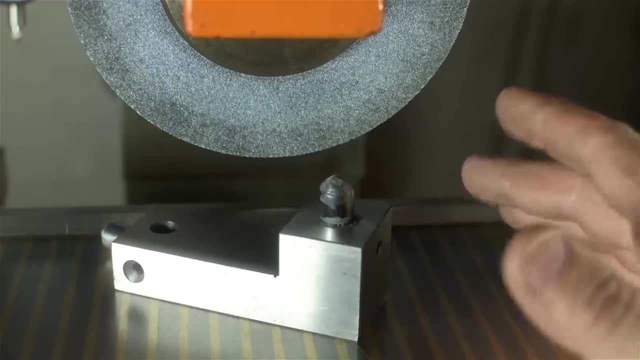 But I know I'd kick myself if I didn't bring this up. This might be the third or fourth time I say this on this channel, When I'm dressing the wheel or when I'm first coming on to a new part that I'm 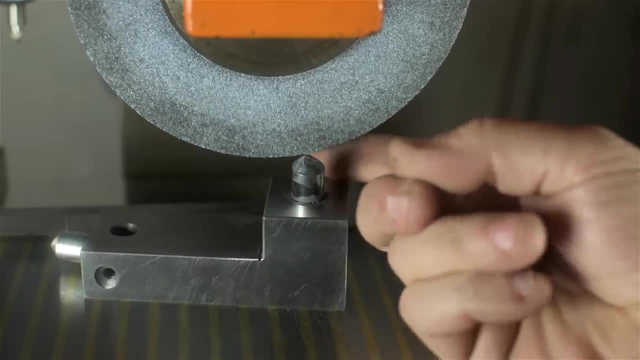 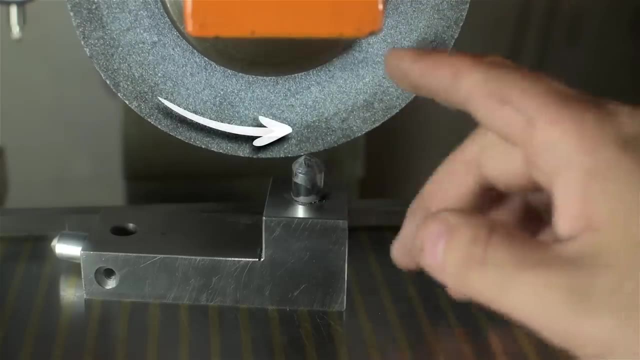 grinding, I always come in from the trailing edge. This grinder spins this way. That might be the opposite from what you're used to seeing. This is an old English grinder with a steering wheel on the wrong side and a wheel that spins the wrong direction. No offense intended to our English. 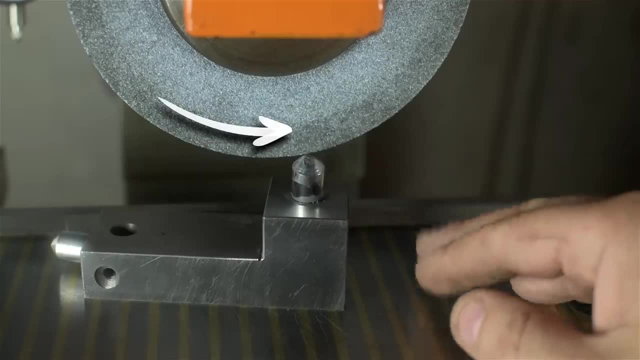 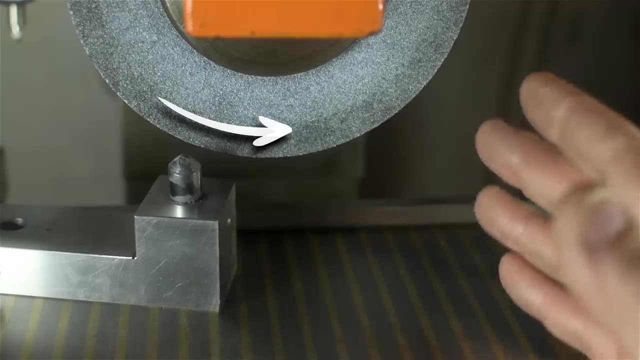 friends out there. Now the grinder itself doesn't really care, but the reason for working on the trailing edge is safety. If I were to work on the leading edge, I wouldn't be able to do that On the left side. in this case, Again, it might be the right side on your grinder If I made some 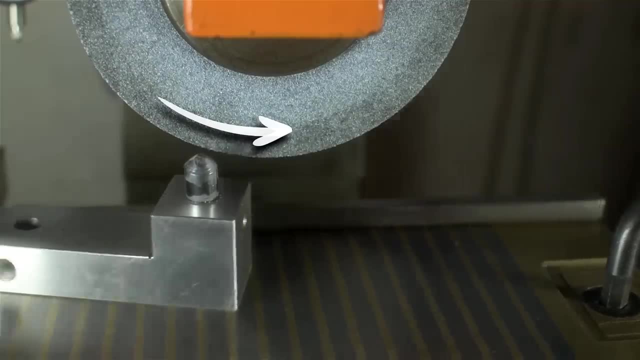 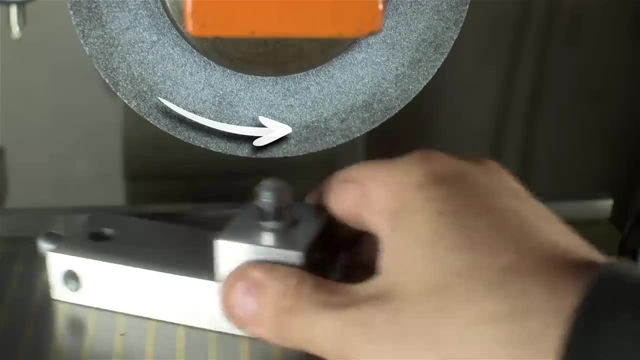 bonehead move with the table while working on the leading edge, it could suck the part or the diamond nib under the wheel. That potentially could be catastrophic If instead I work on the trailing edge. now if I make a bonehead move, I mean it's still dangerous, The wheel could shatter, But the 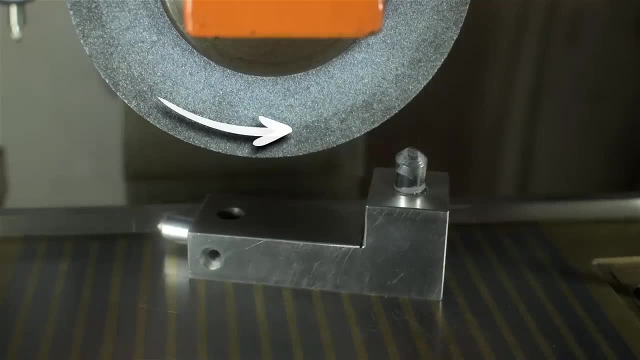 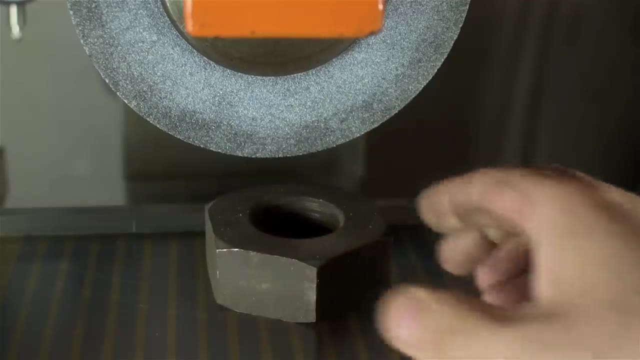 tendency of the grinder would be to kick the part off of the mag chuck and not suck anything underneath it. With that said, let's go ahead and start working on the trailing edge. Let's grind a quick little part and cut to the chase. 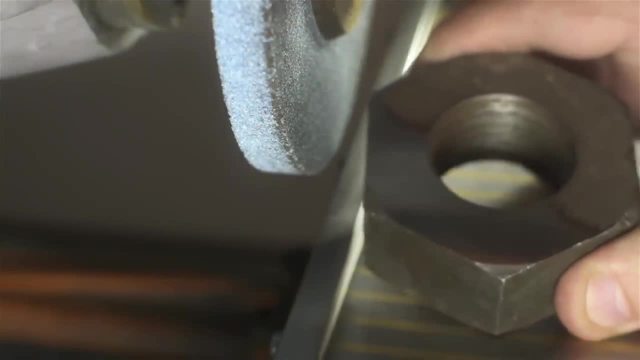 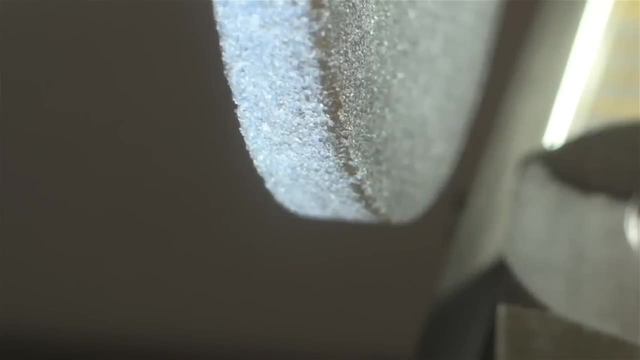 Okay, I think we got a respectable finish there, you know, for rushing through it. No burn marks, at least. But have a look at the wheel. The wear mark- for lack of a better description- is quite small on the leading edge and isn't the whole face. 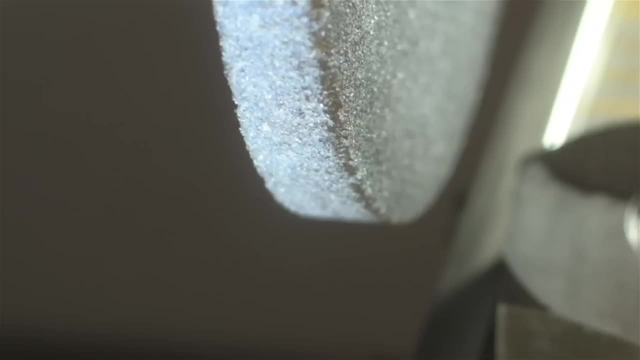 Or edge, I guess, depending on your perspective. when a grinding wheel is used this way, Words are hard. The leading edge is: what does 99% of the cutting or the grinding? The rest of the wheel still looks as fresh as when we faced it Now. granted, this was a small part. 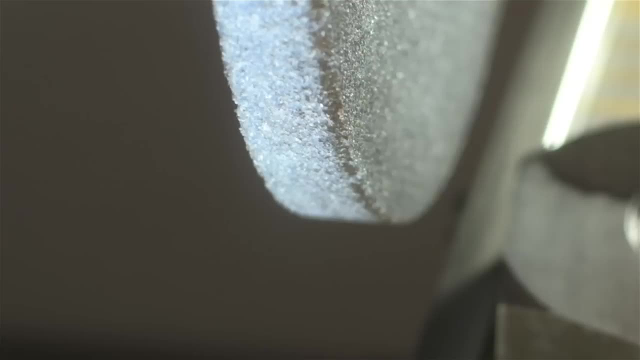 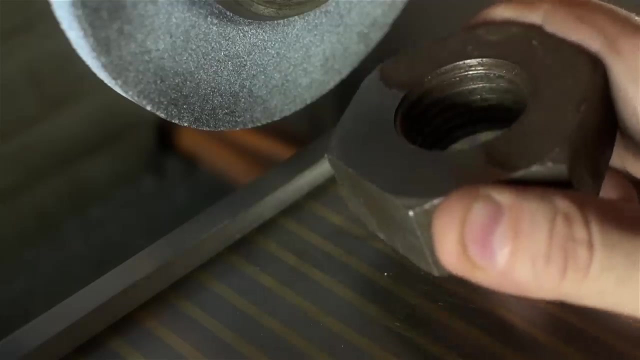 but wear on. the wheel progresses front to back. since we're pushing the part in that way, The rest of the wheel is still there doing final sizing. I suppose, Although the wheel is still breaking down, it doesn't happen as fast as you might expect. I mean, keep in mind we're only 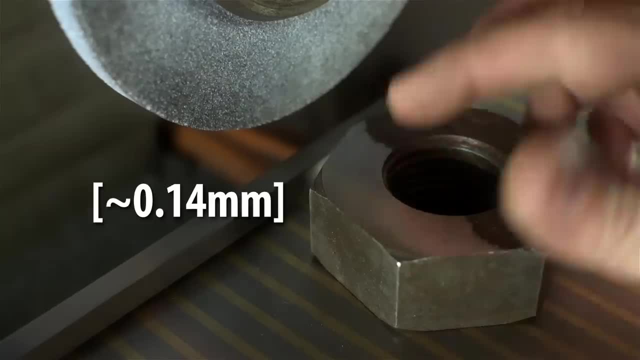 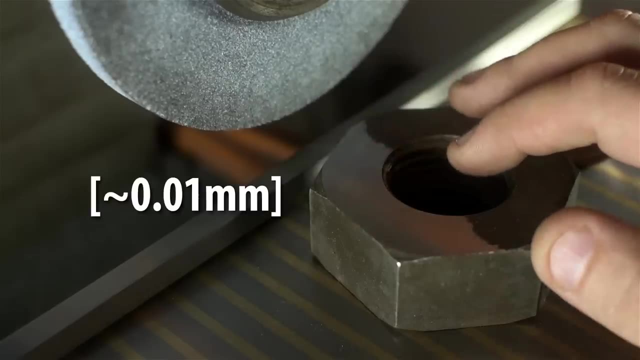 grinding down- I don't know- a few thousandths at a time, Maybe five or six thousandths tops. for this size grinder with no cooling On finish passes that might only be two or three tenths of a thousandth. If you're doing big parts or lots of parts, you do need to dress the wheel every. 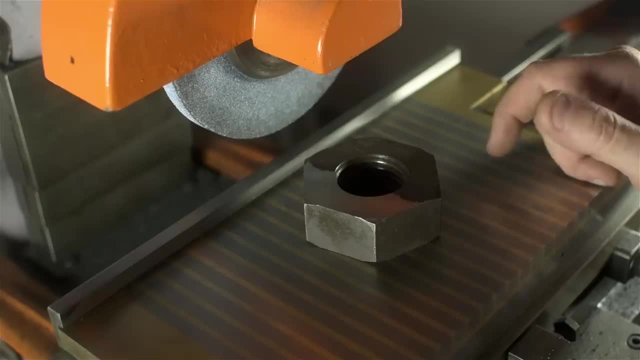 now and again, of course, And dressing the wheel does make it smaller- Not a lot, but remember we're talking tenths on this machine, So picking back up where you left off can be tricky and is part of the black magic that it has. So let's go ahead and get started. Let's go ahead and get.